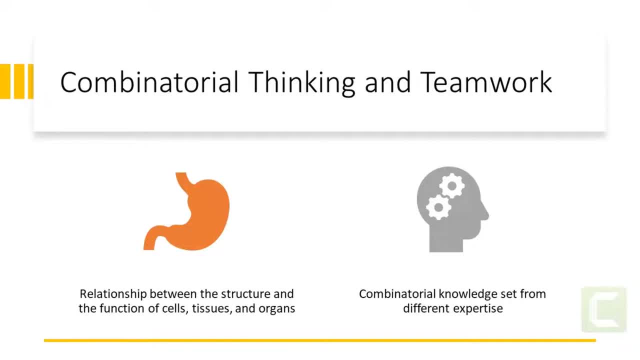 the structure of the tissue and its properties through the suitability for scaffolding is important in order to guide the differentiation and assembly of cells into functional three-dimensional tissues. This builds upon knowledge how molecules perform in terms of their bioactivity when embedded within engineered tissues to assist in accelerated healing processes upon surgical implantation. 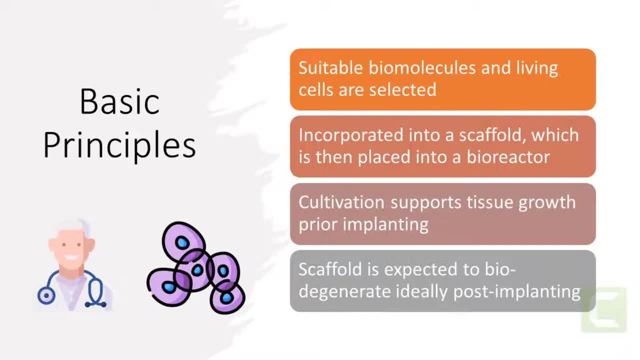 In a classical tissue engineering approach, living cells and biomolecules are incorporated into a scaffold, which is then placed in the tissue engineering process. The tissue engineering process is then incorporated into a scaffold, which is then placed in the tissue engineering process. The tissue engineering process is then incorporated into a scaffold, which is then placed. 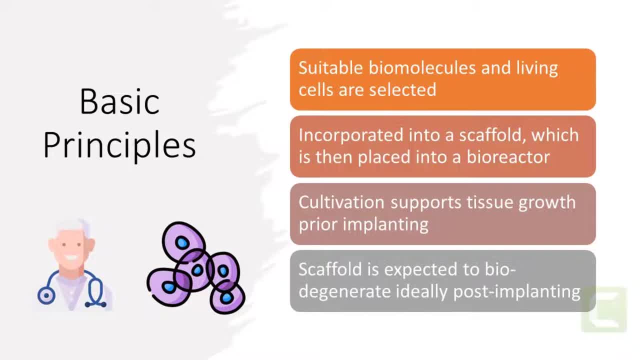 into a bioreactor. Cultivation within the bioreactor in vitro allows engineered tissues to reach some degree of function before they are implanted. In the ideal case, cells grow and start to make tissue within the scaffold. The scaffold is expected to supports further cell function proliferation. 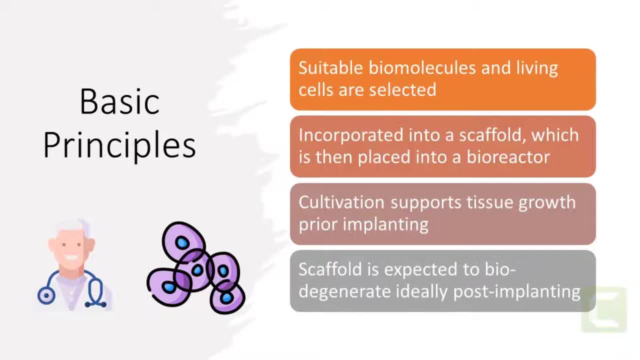 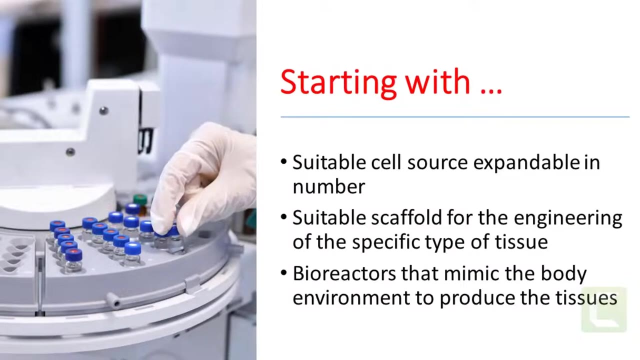 or differentiation and allows blood vessels to infiltrate, while the scaffold itself biodegrades. once this engineered construct is implanted into the body, This is where the cells differentiate into the desired tissue and the tissue starts performing its proper function. Tissue engineering requires the following to work upon: It requires a cell source expandable. 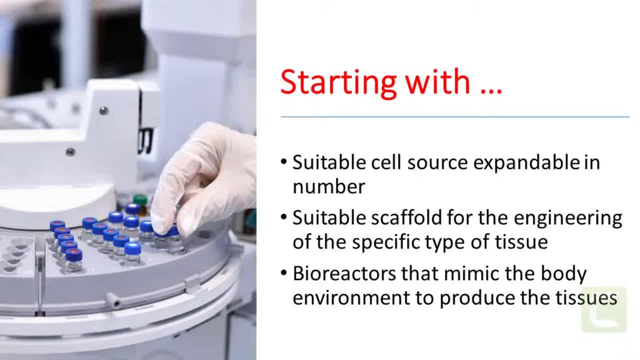 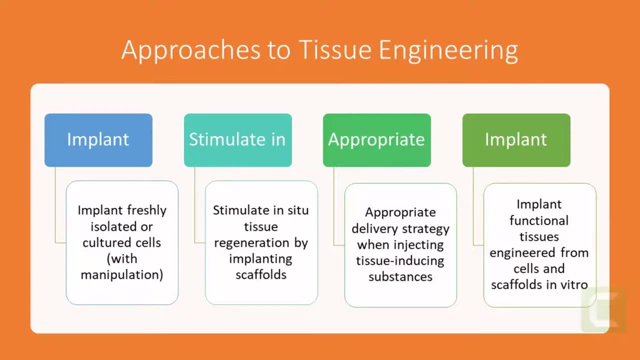 in number, followed by a scaffold that is suitable for the engineering of the specific type of tissue and scalable bioreactors that mimic the body environment for the production process. There are three main approaches to tissue engineering. The first is to implant freshly isolated or cultured cells to treat diseased or injured. 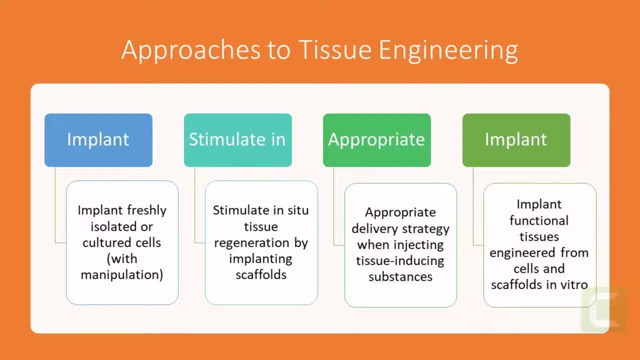 tissues. Cells can be manipulated to suit a patient's needs before implantation. The benefit of doing so is that cell implantation eliminates complications and morbidity associated with surgical procedures, though concerns exist if the cells being washed out from the site of injection or issues regarding the inability of the implanted cells to maintain proper function. 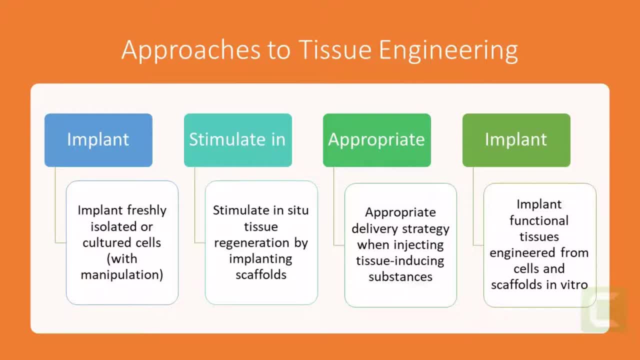 The second strategy is to stimulate in-situ tissue regeneration by implanting scaffolds or injecting tissue-inducing substance at the injured tissue. This method requires purification of the tissue-inducing molecules as well as selection of appropriate delivery methods, ie controlled delivery. 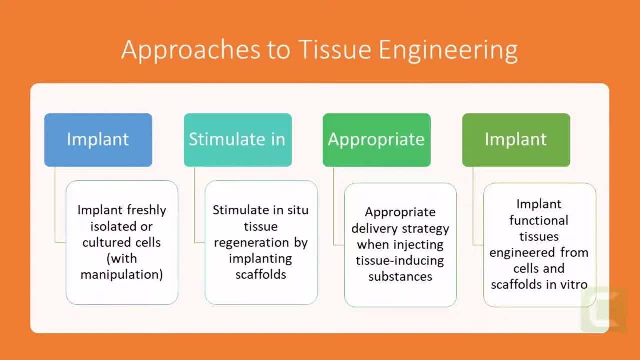 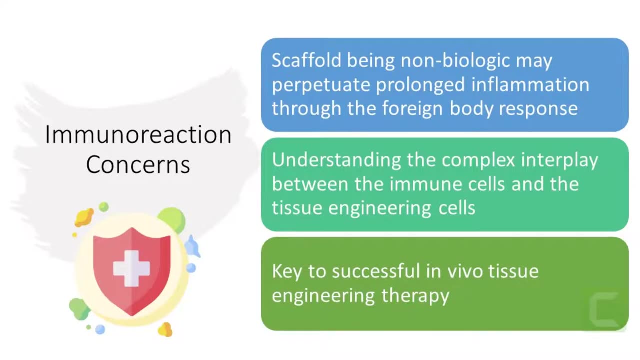 soluble factors. The third is to implant functional tissues engineered from cells and scaffolds in vitro. This requires optimization of cell ratio and density, as well as mechanical and biochemical properties of scaffolds. All the approaches discussed above can lead to immunoreaction, depending on the cell source and 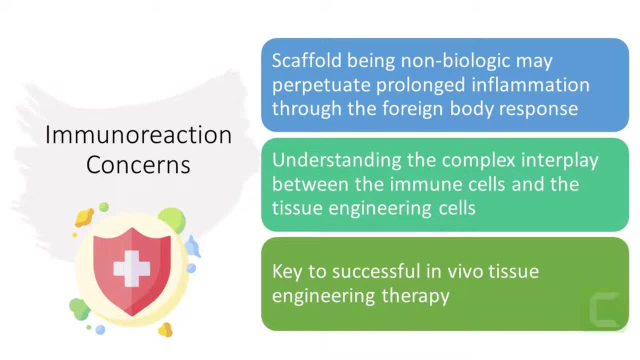 the type of biomaterial used. Implantation of cell-laden scaffolds is a promising strategy for regenerating tissue that has been damaged due to injury or disease. However, the act of implantation initiates an acute inflammatory response If the scaffold is permanently damaged. the implantation process is a promising strategy. 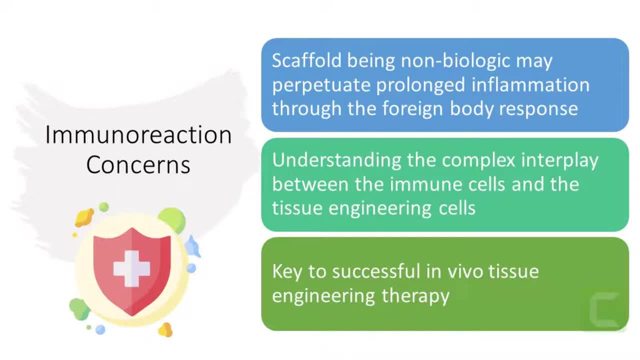 In the case of cell implantation, the implantation process is a promising strategy. If the scaffold is constantly damaged, the implantation process is a promising strategy is nonbiologic inflammation will be prolonged through the foreign body response, which eventually forms a fibrous capsule and walls off the implant from the surrounding host tissue. 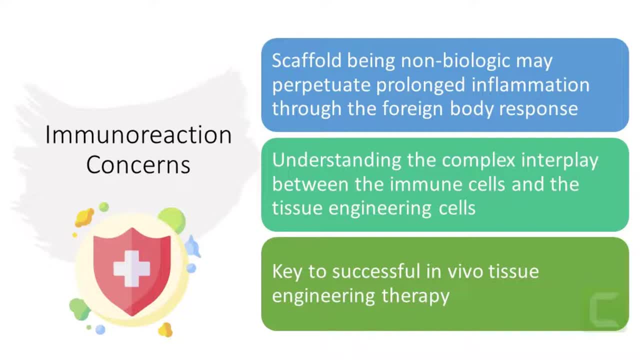 This host response from a cellular perspective can create a harsh environment, leading to long-lasting effects on the tissue engineering outcome. At the same time, cells embedded within the scaffold can respond to this environment and influence the interrogating immune cells, such as macrophages. 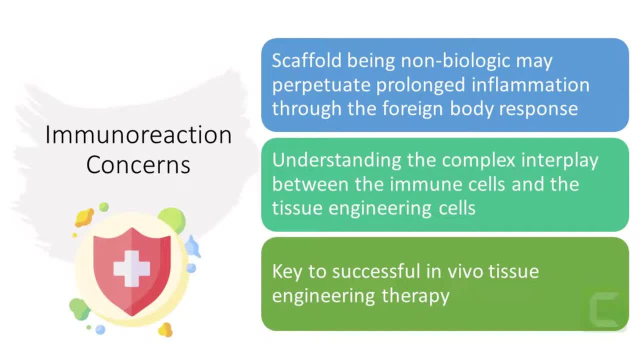 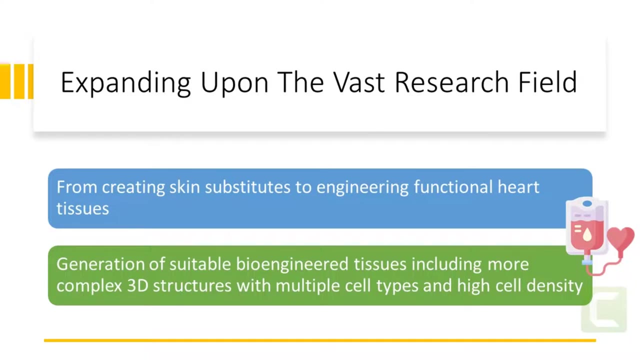 Understanding this complex interplay between the immune cells, notably macrophages, and the tissue engineering cells is a critically important component to a successful in vivo tissue engineering therapy. Since then, tissue engineering has rapidly grown into a vast research field that has studies ranging from creating skin substitutes to engineering functional heart tissues. 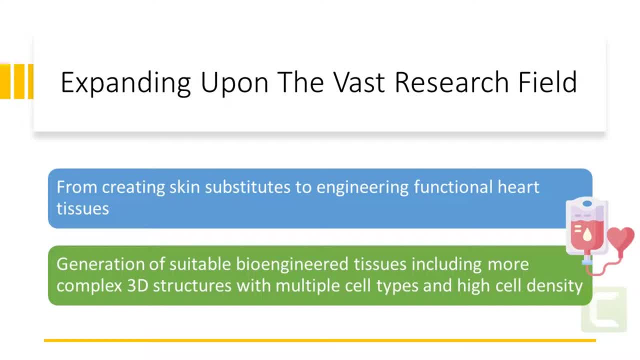 Engineering of skin nerves, bone, bone marrow, cartilage, blood vessels, corneal epithelia, arteries, heart valves and heart myocardium are among the many current research areas in tissue engineering. The past decade have revealed advances in our understanding and generation of suitable 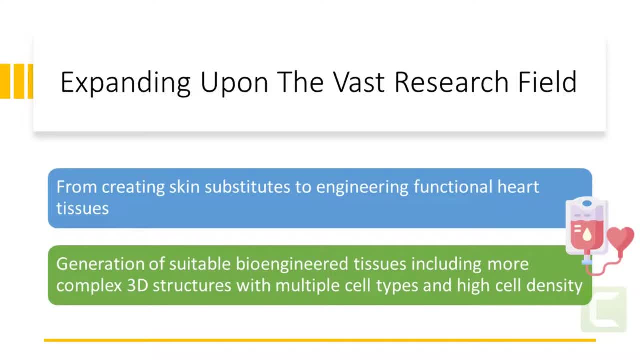 bioengineered tissues, including vascular prostheses, infection caused by biomaterials, skin and connective tissues and functional tissue transplants. Much progress have been made from initial two-dimensional tissue layers towards more complex tissue structures such as the blood vessels or myocardium are more difficult to.